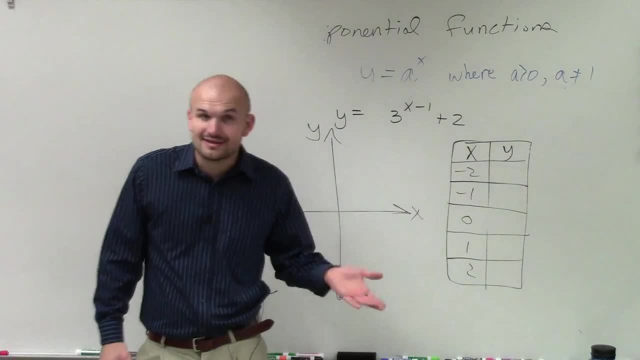 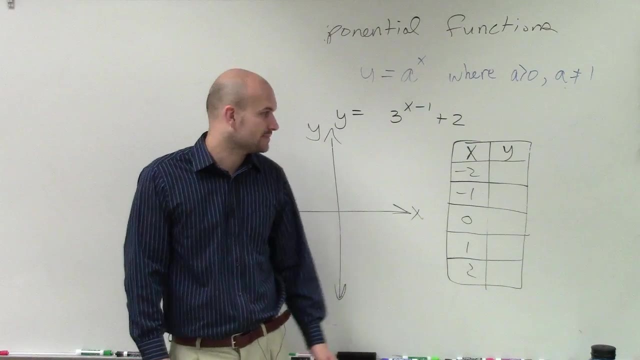 0,, 1, and 2.. That way, I got some negatives, I got some positives and we got the best number in the world- 0, as well, Because that's always nice to calculate with 0.. So now remember if I have an. 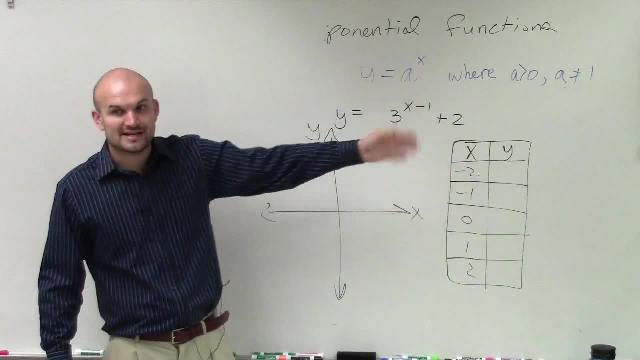 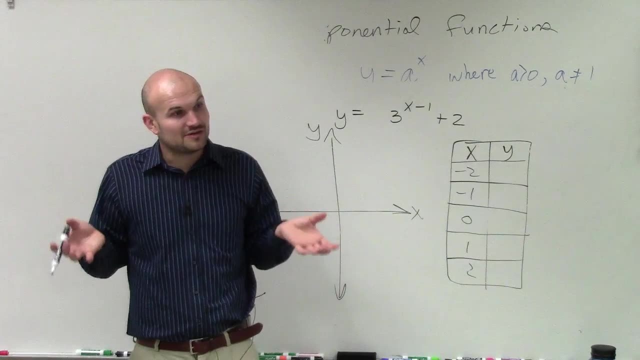 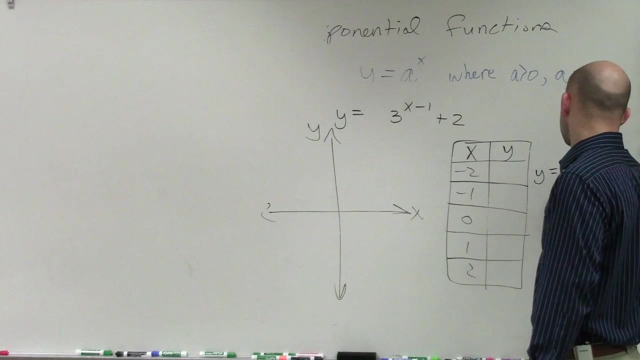 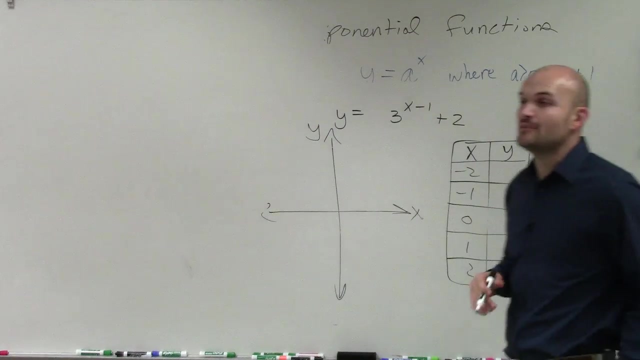 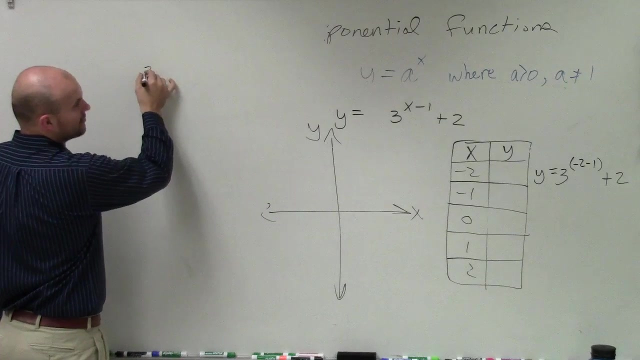 equation: if I have the x value, I just plug in the x value to find the y value. Then I have an x and a y coordinate, or x and y. I have a value. so therefore I have a coordinate point which I can plot. So negative 2.. So I have y equals 3 times negative, 2 minus 1 plus 2.. Well, negative 2 minus 1 is going to be negative 3. So I have 3 raised to the negative third plus 2.. 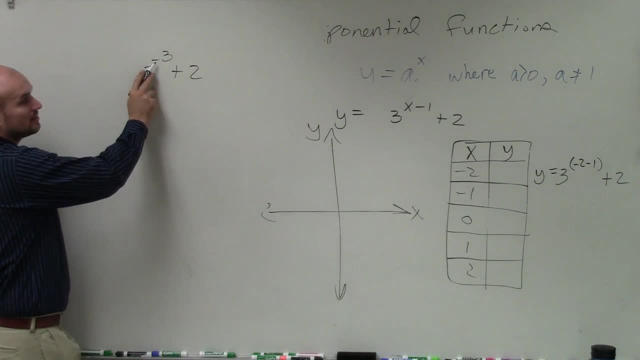 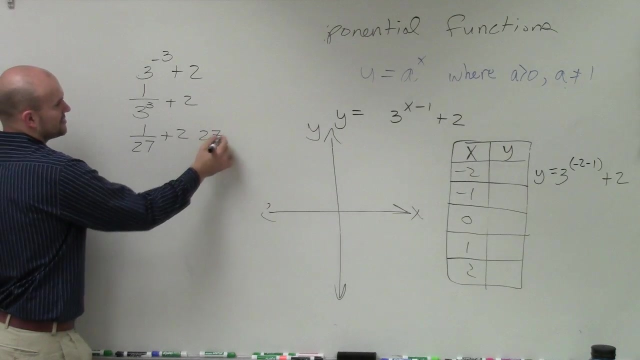 So now, remember 3 to the negative. third, remember that's a negative. So that's the same thing as 1 over 3 cubed plus 2, which is 1 over 27 plus 2, right, Then make those the same fractions. 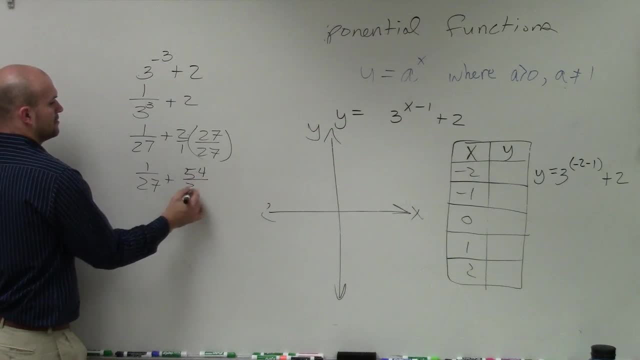 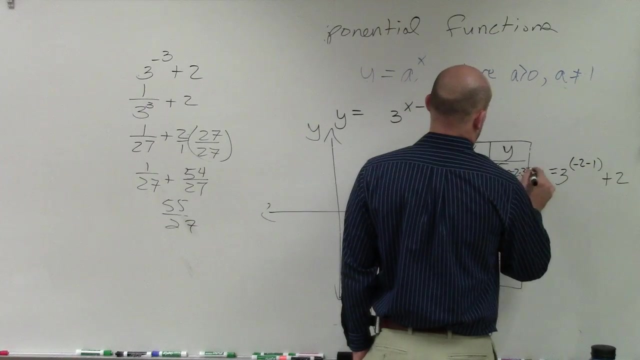 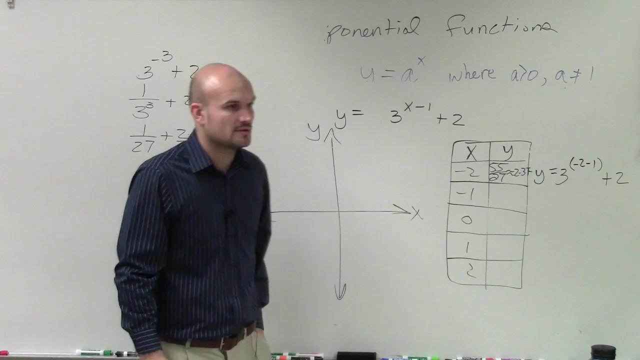 That's going to be 54.. So 54 over 27 is what? What is the decimal? So you could say 55 over 27, or obviously, if you're going to be graphing, it's like 2.37,. they said approximately 2.037.. Okay, so it's almost at 2, then. 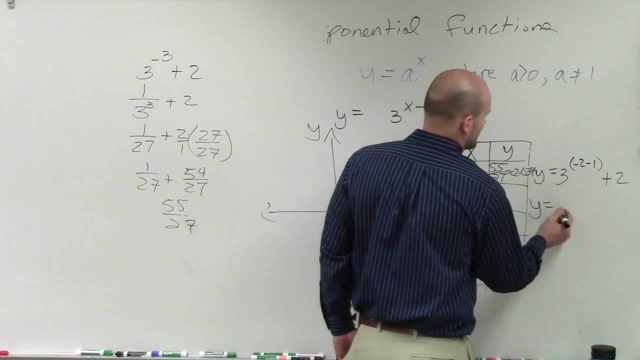 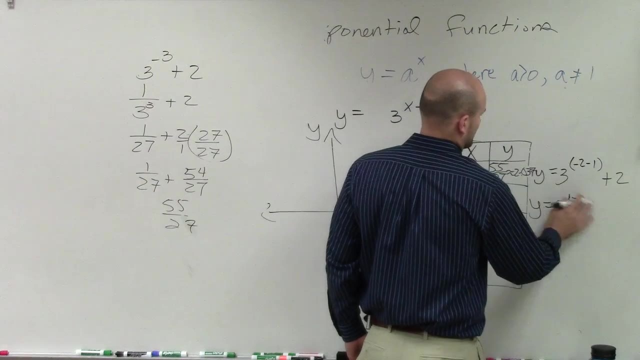 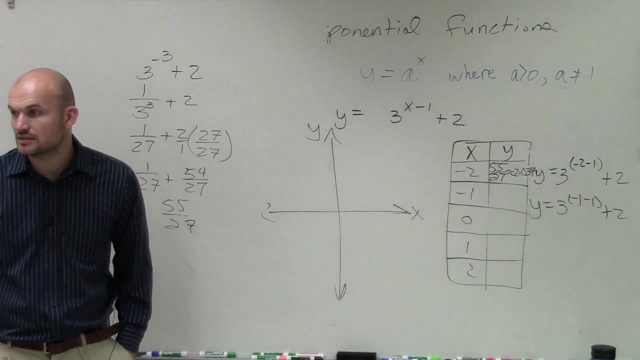 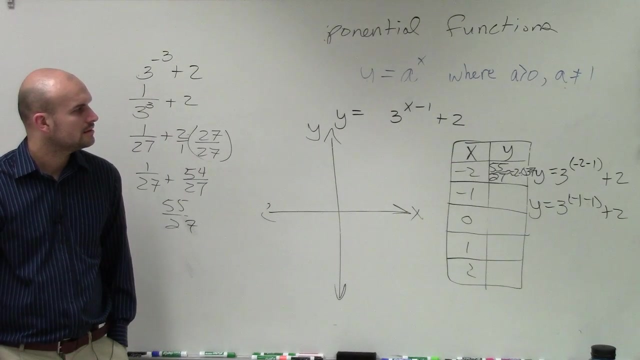 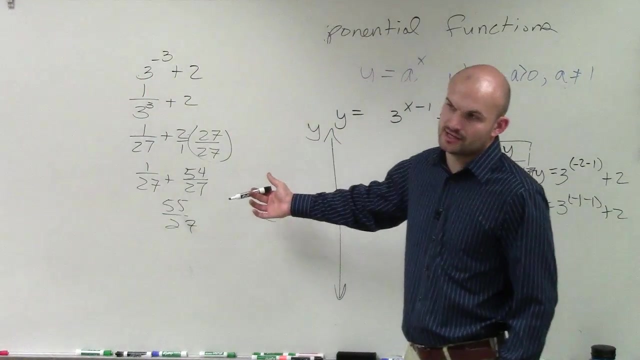 All right, so now let's do negative 1.. So I just plug in 3 times: negative 1, negative 1, minus 1, plus 2.. Yes, Yes, You could, but then you're not going to know what any of the behavior is on the negative side, right? 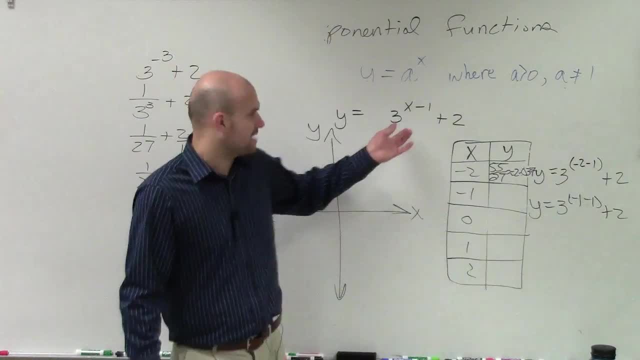 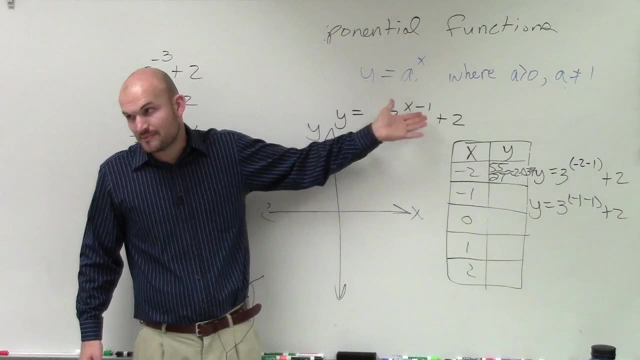 So I was kind of more talking about fractions when I have a fraction as my A. but again, still, yeah, you're not really going to be able to, you could probably, we could probably pick different numbers. that might be a little bit easier with this, but it's okay. 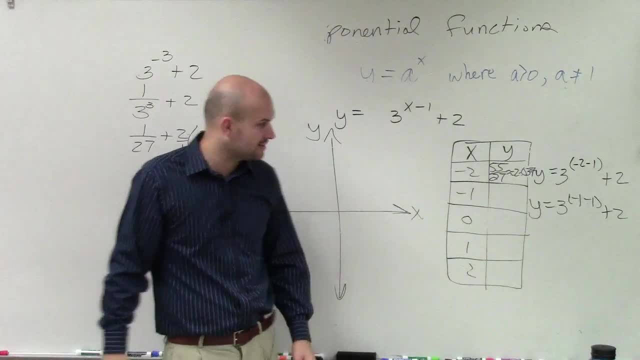 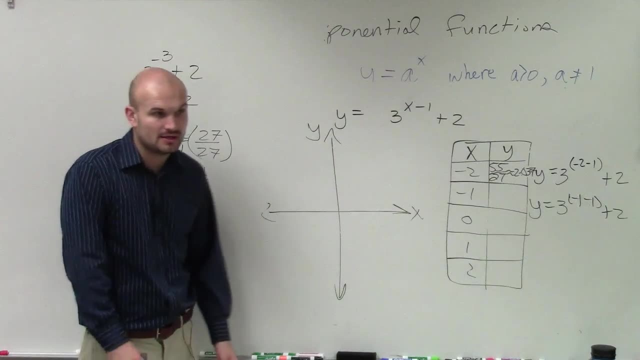 You can use decimals for this graphing. This is just a basic you know kind of thing with this. So therefore I have 3 over negative, 1 minus 1, which is 3 to the negative. second power right, which is 1. ninth, 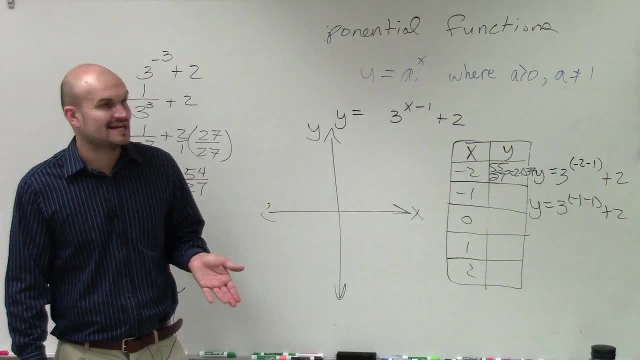 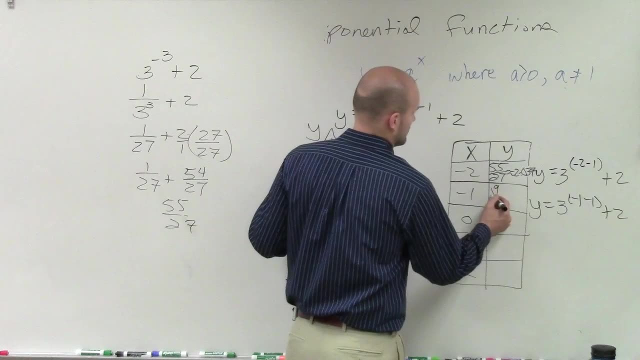 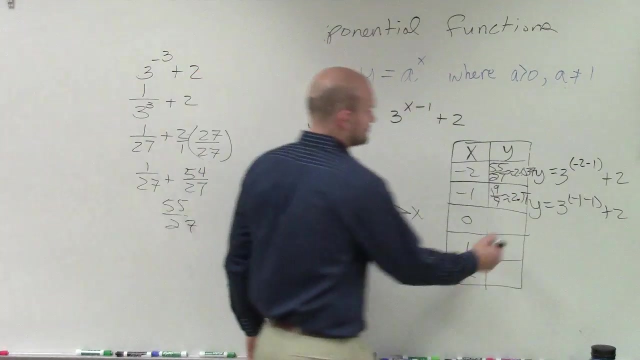 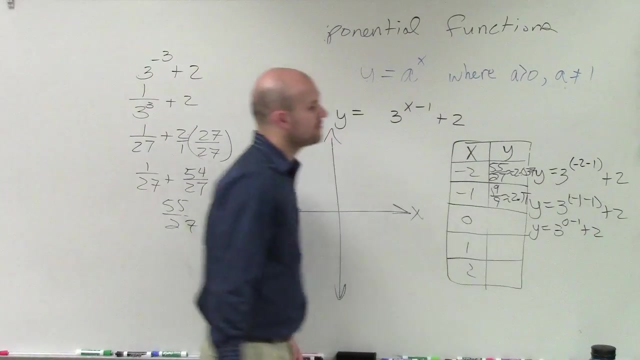 1, ninth plus 2 is going to be 19 over 9.. Yes, 19 divided by 9 is Anybody Okay? And then let's do 0. Ah, decimals. So I have 3 raised to the 0,, 3 raised to the 0 minus 1, which is 3 to the negative first power. 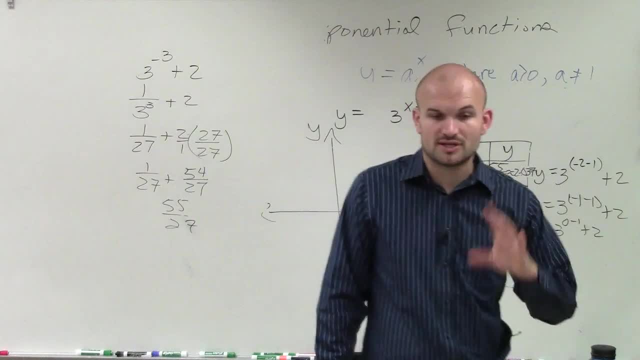 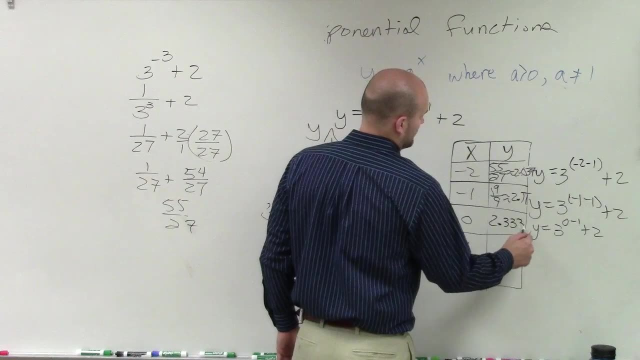 So 3 to the negative first power is 1 third. 1 third plus 2 is going to be 4 thirds, Which is 2.333.. All right, Now let's get to the easier answers. That's 4 thirds. 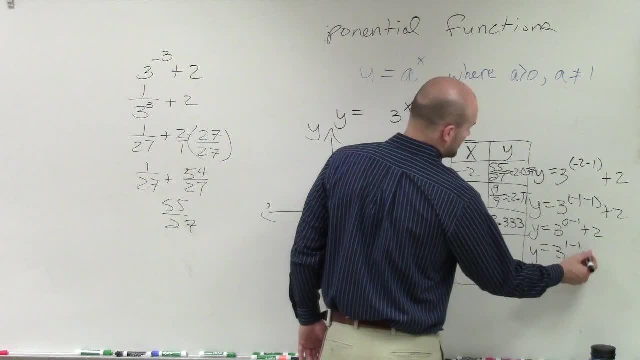 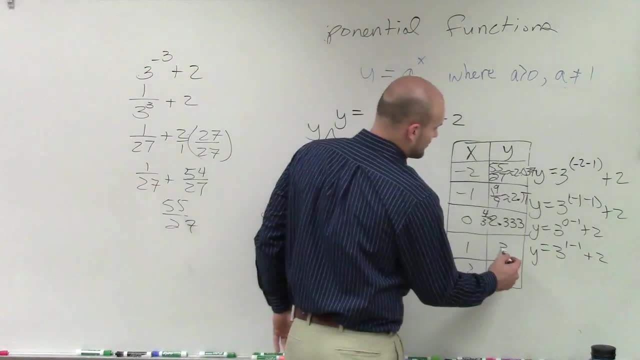 So y equals 3 to the 1 minus 1 plus 2.. Well, 1 minus 1 is 0.. 3 to the 0, power is 1.. 1 plus 2 is 3.. And then I have 2.. 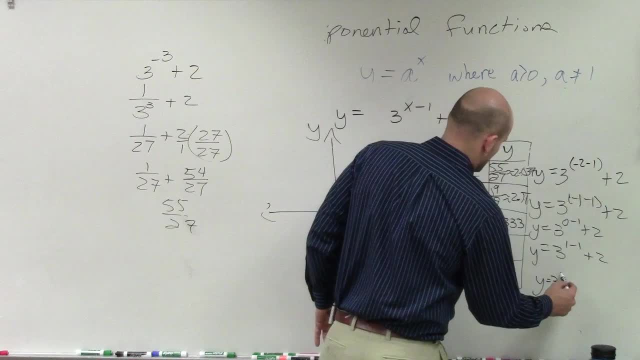 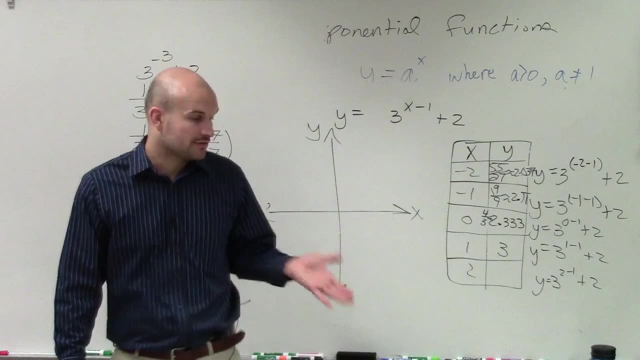 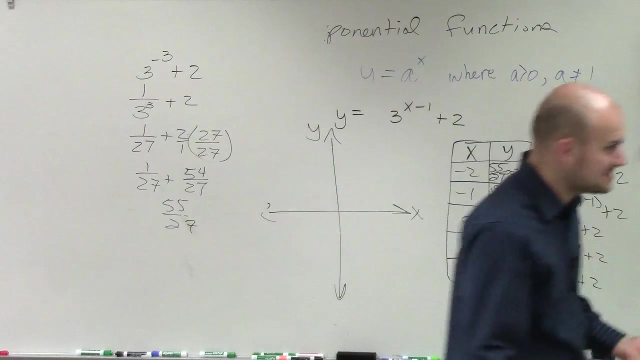 y equals 3.. 3 to the 2 minus 1 plus 2.. 2 minus 1 is 1.. 3 to the first power is 3. Plus 2 is 5.. All right, So again, ladies and gentlemen, I'm just going to be estimating with this table. 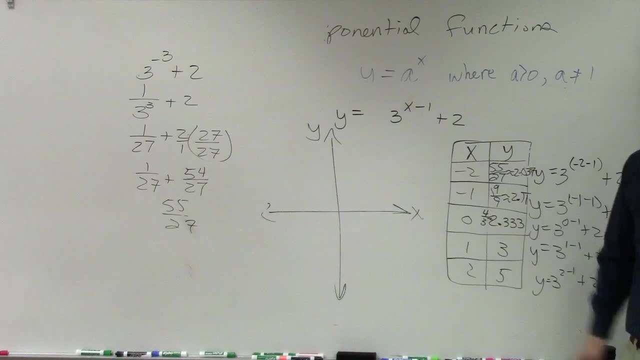 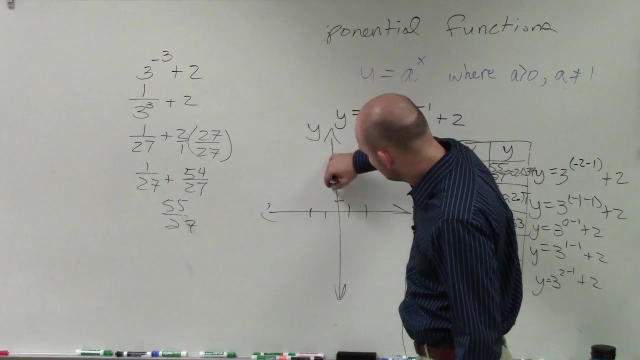 There's other ways we can go through this, But I just want you guys to understand. you can always plug in your values, All right, So let's go at negative 2.. And negative 2, we said it was around What. 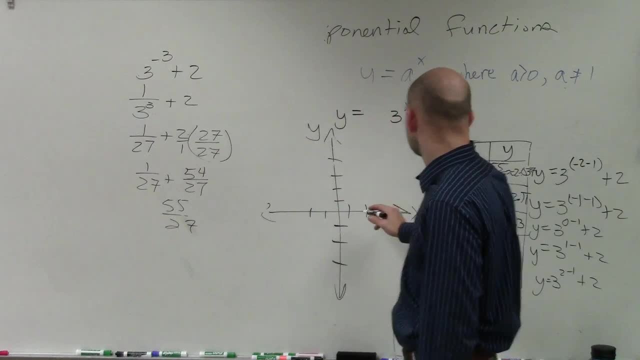 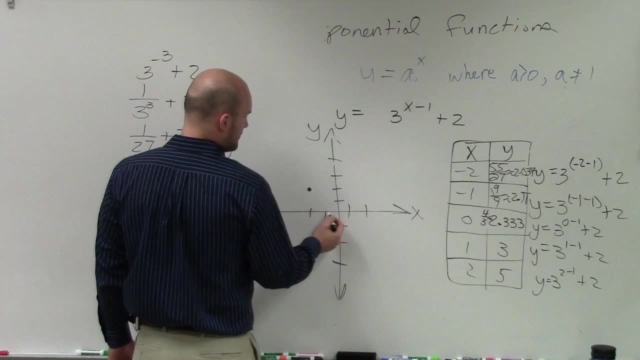 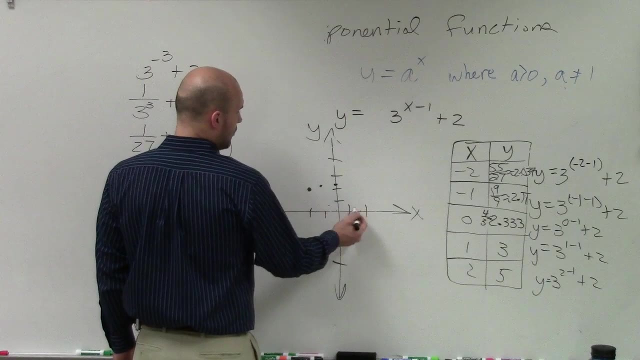 So at negative 2,, we're just over 2.. At negative 1,, we're a little bit higher. At 0,, we're at 2.33.. At 1,, we're all the way up to 3..